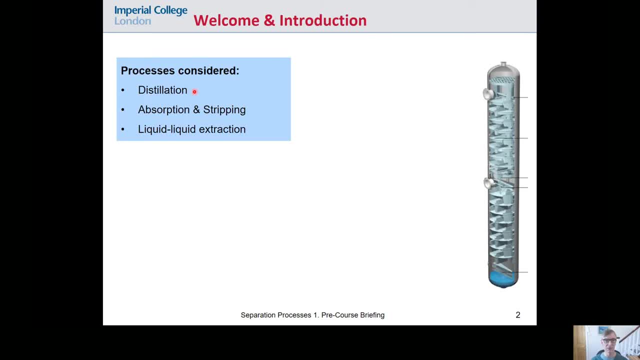 specific processes and their distillation. I guess you're familiar with distillation. we'll restrict this to mixtures of just two substances and it'll be continuous distillation. Two other related processes are absorption and stripping. Absorption is where you have an 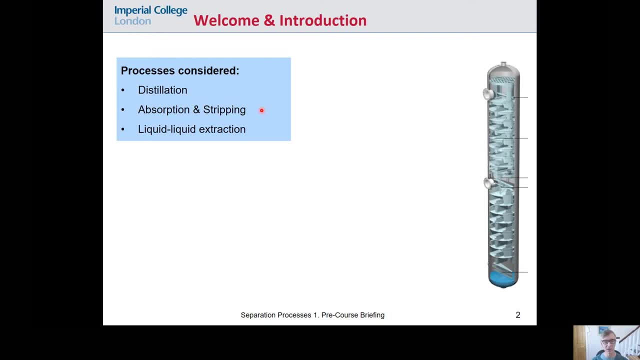 impurity in a gas and you absorb it into a liquid. Stripping is the reverse, where you have an impurity in a liquid and you want to extract it or strip it out using a gas, And then, finally, we'll look at liquid-liquid extraction or solvent extraction. 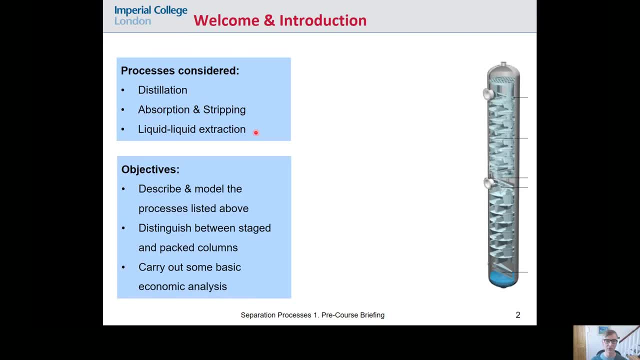 which is a process you may be familiar with. The objectives of the course are really three. The first is to be able to describe and model the processes I just listed. Model means essentially that you can carry out quantitative design calculations to, for example, design a distillation. 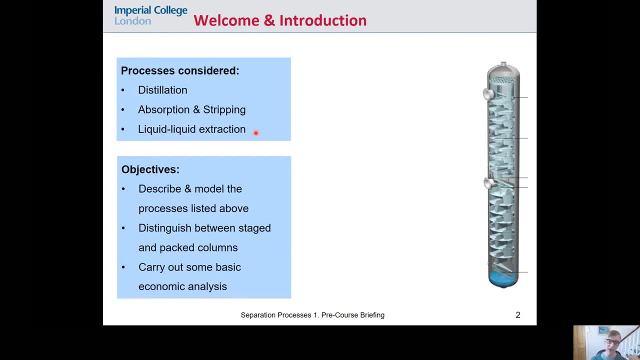 process that would work. We need you to be able to distinguish between staged and packed columns- so that's something you'll come to learn about in the course itself- and to do some basic economic analyses. So those are really the three things that you need to be able to do by the end. Where does 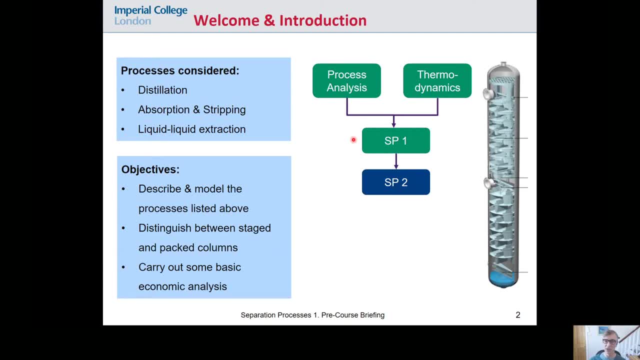 it sit Well. as I said, it's a first-year course. It's taught actually in the second term, the spring term, and it draws on material that you will study in the first-term process analysis course, which is mainly around energy and material balances, which are absolutely fundamental to the 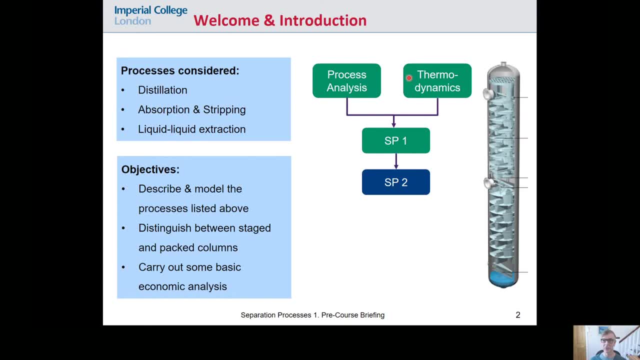 separations. You'll also draw a little bit on the thermodynamics course, which is also a first-year course, And in year two you'll do separation processes too. so that's the connection between the courses In terms of the structure. we'll have a 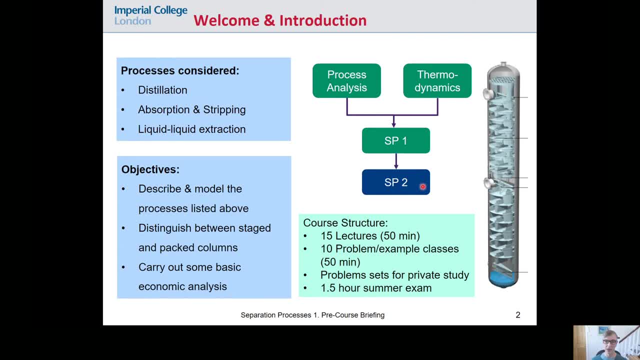 three-year course and we'll have 25 timetabled slots. They're an hour, but normally the class lasts 50 minutes. I will do all of these live either on Microsoft Teams or, if conditions allow, in person in the lecture theatre, And I'll use the 25 divided between lectures, around 15 lectures. 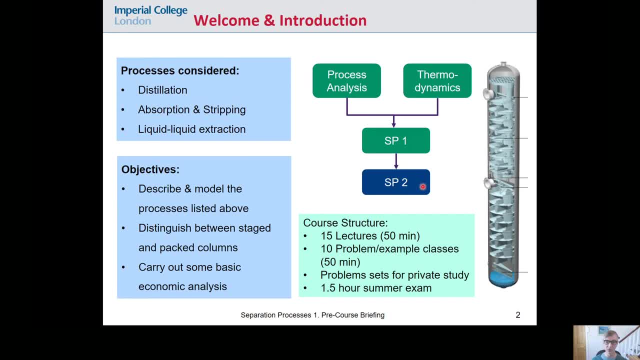 and 10 problem or example classes And I would like you all, as students, to you know, to log in, even if it's remote, to log in and take part. You can do that live in the class and I really welcome questions. They're very important.